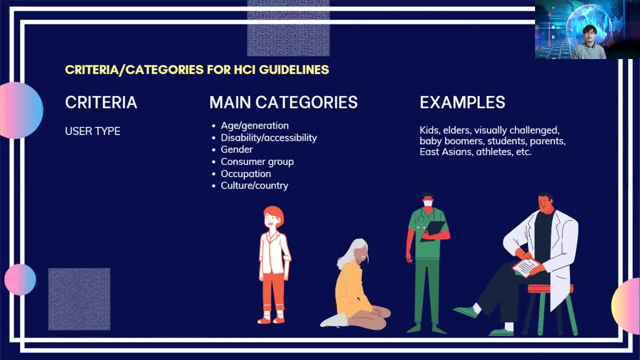 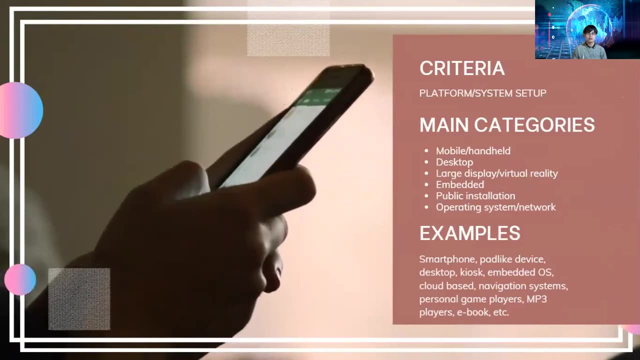 to create a system, you must identify the user type or who will going to use your system. Okay, so that is our first guideline: Know the user type, know the user who are going to use your application. Okay, Next criteria, is okay with me. 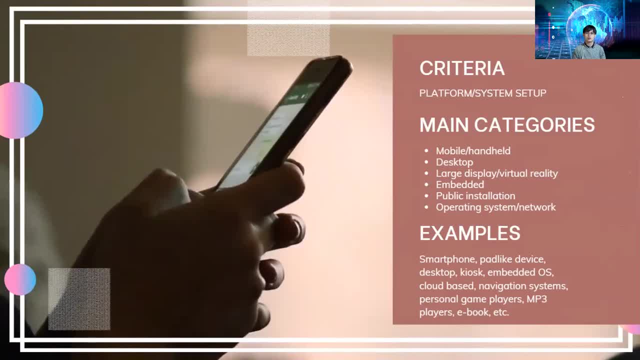 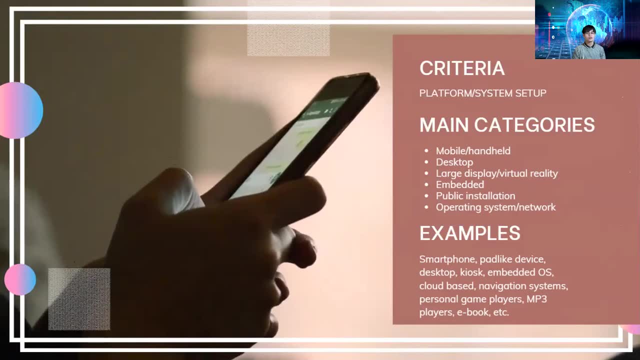 Yeah. Next criteria is the platform or system setup. After knowing who will going to use your system, you must know what, which platform or what would be the set of your system. Okay, so it categories involves: would it be mobile or handheld? 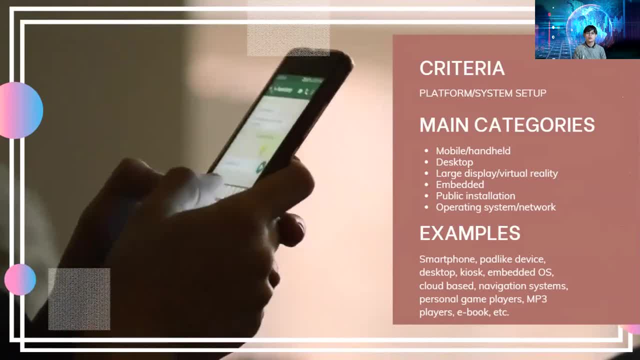 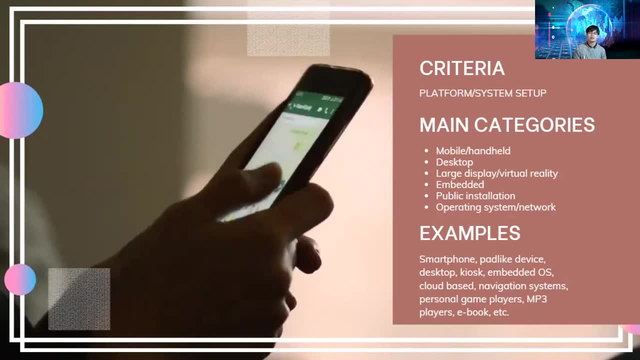 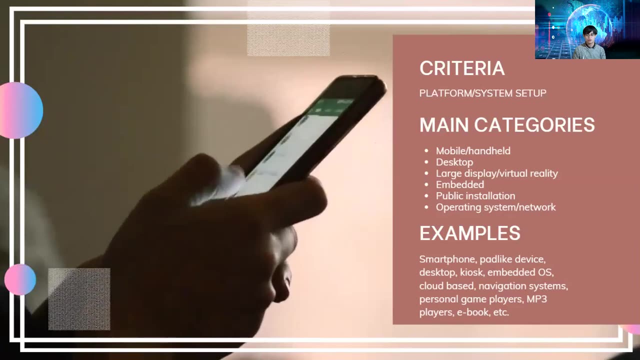 Would it be desktop application, or would it be a large display of virtual reality, or it be embedded, or public installation, or operating system or network? so you must identify the setup of your system, okay, so examples for that would be smartphones, pod-like device, desktop chaos, embedded OS, cloud-based navigation. 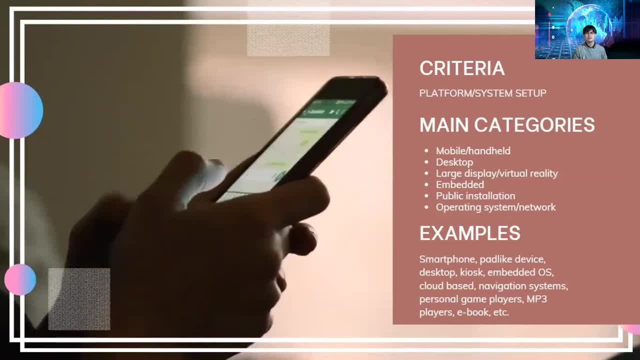 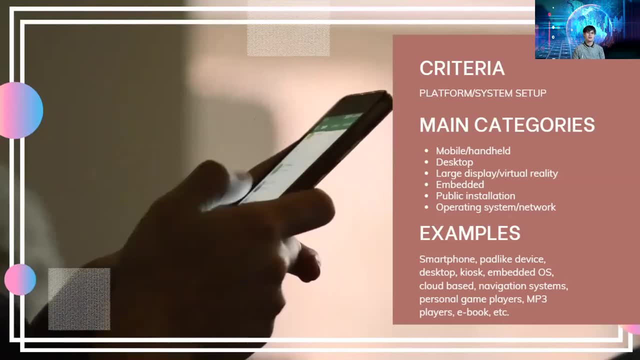 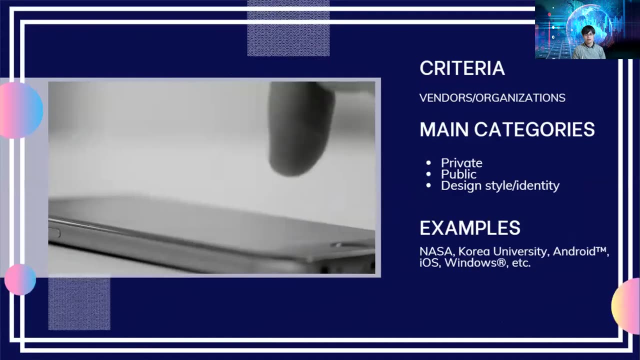 systems, personal game players, queue systems and etc. so this is very important: that you should know what would be the system of your system, okay, before creating a really good HCI design. okay, and next for that next criteria: the vendors or the organizations. okay, so the main. 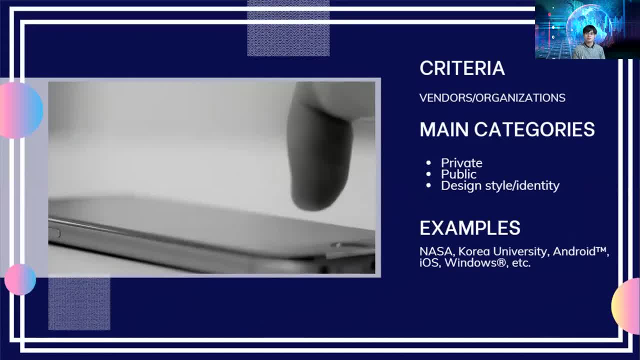 categories involves: is it in the private, public, or design, style or identity. so examples for that would be NASA or Korea University. is it for the Android? is it for the USPP? is it in iOS, Windows? so you must know the organization, you must know the vendors. okay, that's one of the most important thing. also, before, 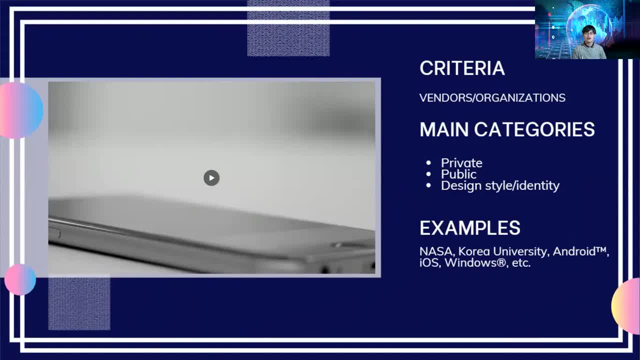 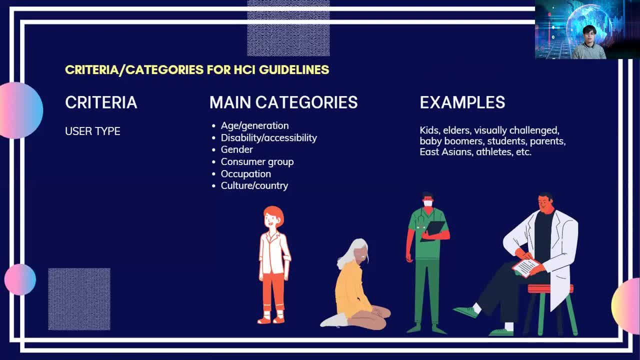 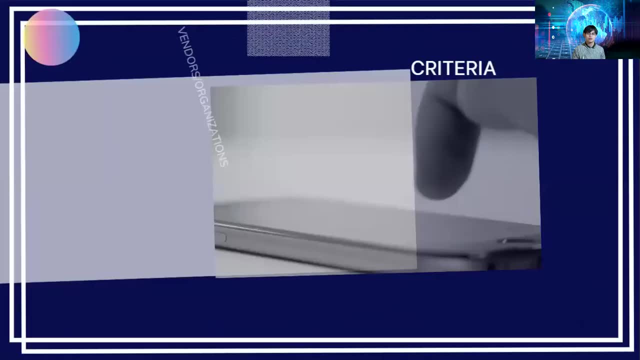 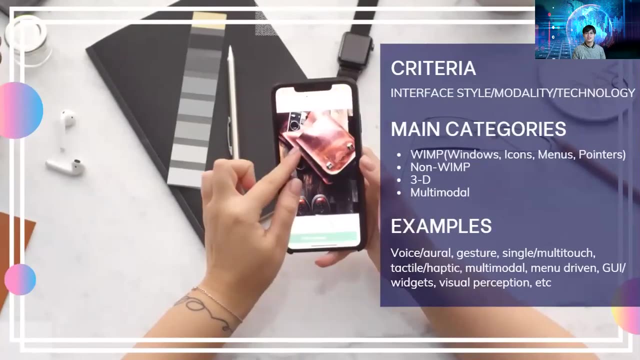 creating a good system. okay, again, first that we need to consider is the user type. next is- let me go back again- the user type, the platform or the systems set up, and the third is the vendors organization. and the fourth one is the interface style. okay, the modality, the technology is it? 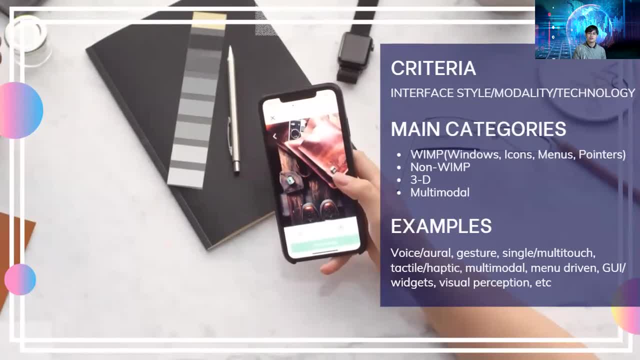 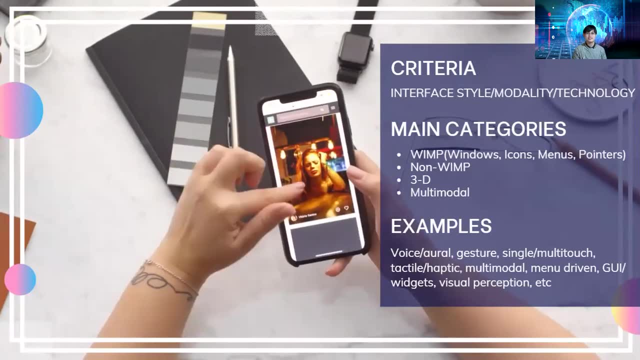 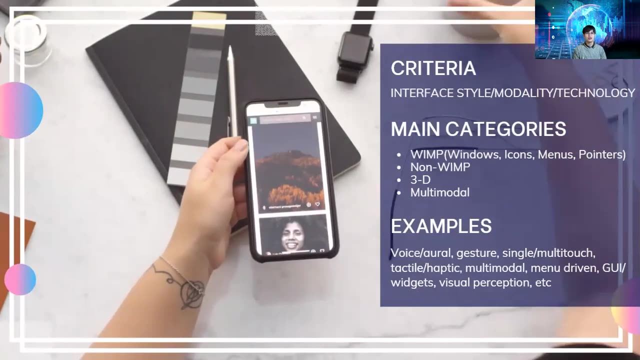 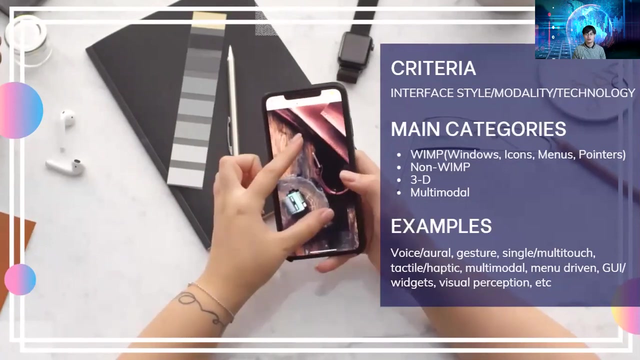 is it open? will it involve window icons, menus, printers or nanWWEB, or is it in 3D for multi-modal? so it's kind of very, very important also to consider that we need to know the interface style. okay, so the interface style, the modality and the technology examples with that. 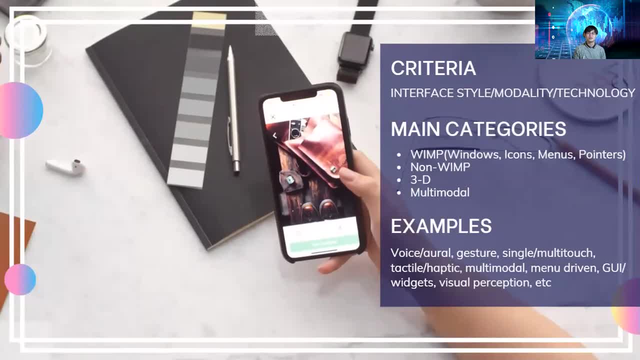 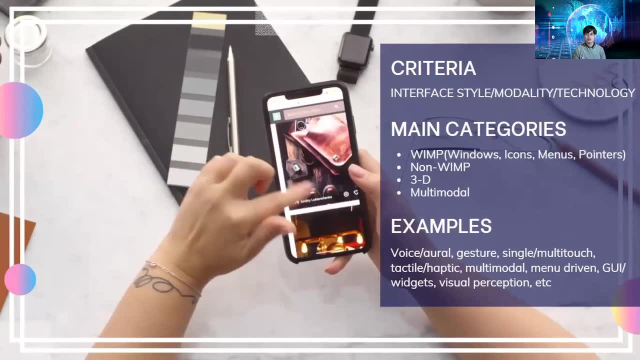 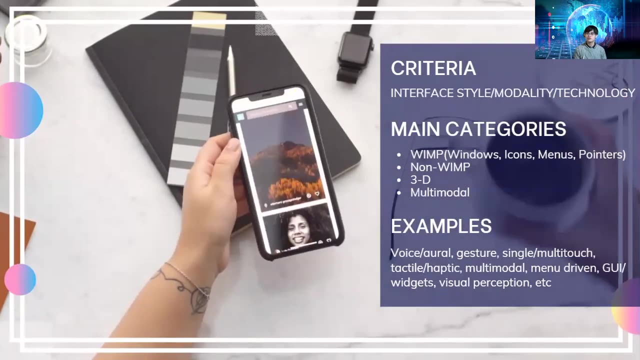 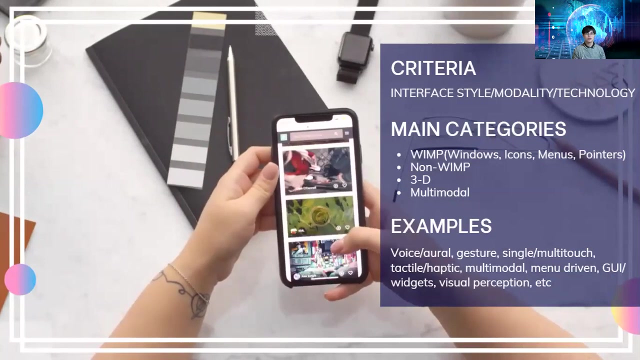 would be voice or oral. the application that's this: voice features, voice command feature, the gestures, this thing, is it single or multi touch, tactile or haptic, multi-modal menu driven going, or does it a widget? visual perceptions and etc. it's very important also that when designing a really good SCI, you must 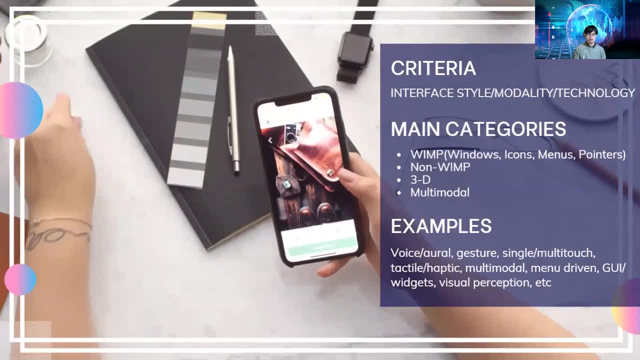 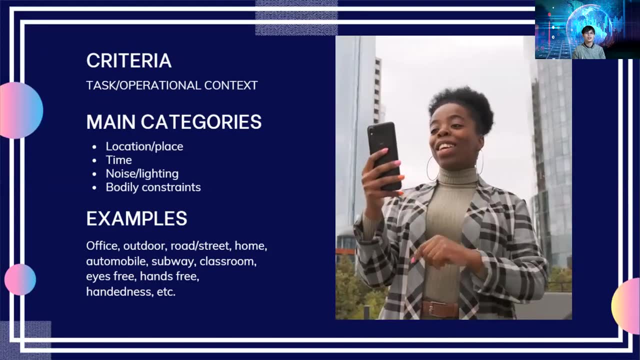 know the interface style. okay, let's move on with the next criteria: the task or operational context. so again, in the previous presentation I have discussed that when creating a web application, you need to know the interface style. okay, let's move on with the next criteria: the task or operational context. so again in the previous presentation I have discussed that when creating a web application, 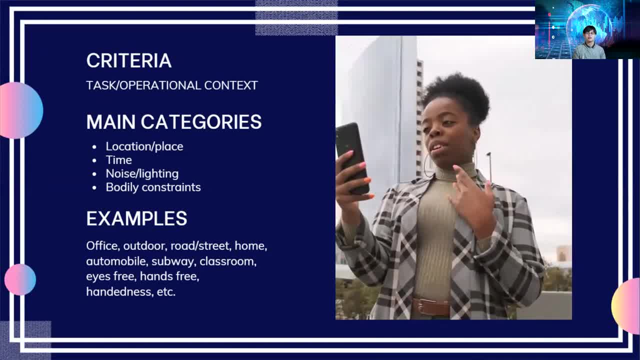 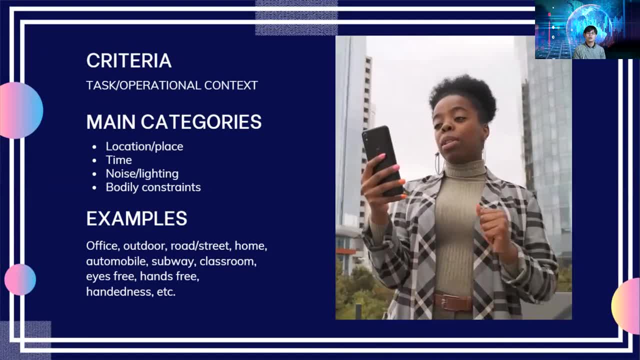 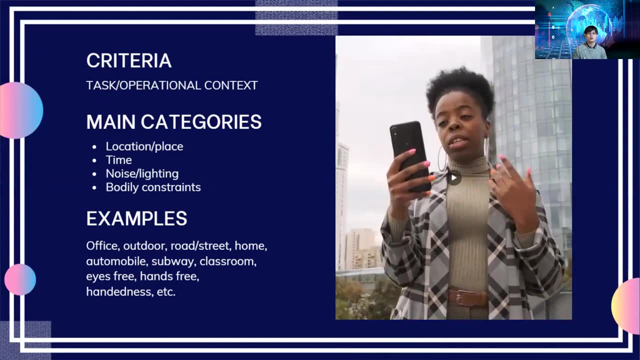 a system, you must identify the different jobs or the different tasks, or what are the different features that your system will going to do, how it will gonna solve the problem. okay, so for the task or the operational context, the main categories involve the location or the place, the time, the noise, lighting. 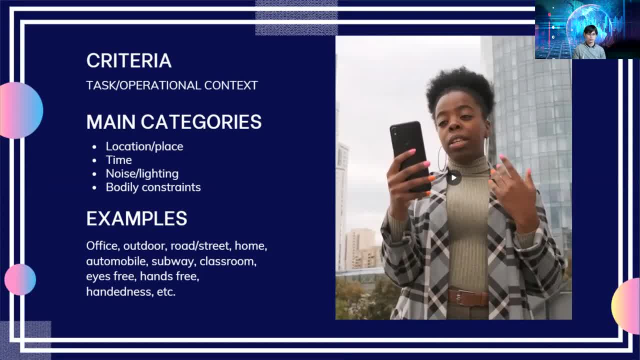 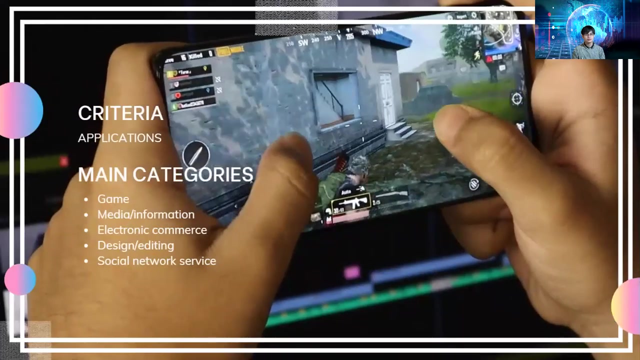 federally constrained. okay, for example, that would be office, outdoor road, or see home, automobiles, subway. is it for the classroom? is it ice, ice free and three handed man's and etc. it's kind of very important that we should and identify all the tasks, all the jobs that your system will be to do. okay, next, next. 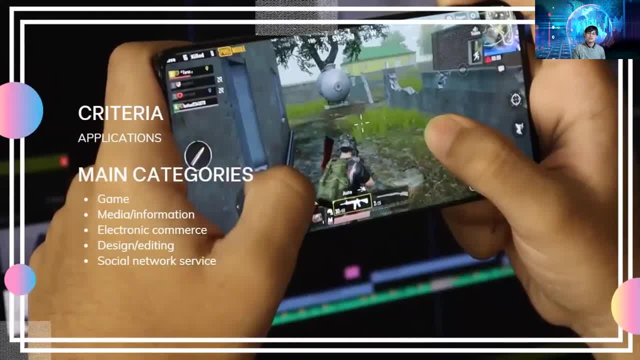 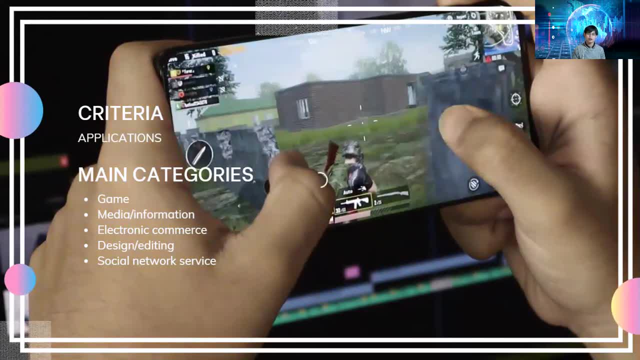 criteria: application. what kind of application would that be? is it a? is it for the gaming? is it a game application? is it a media or information? is it electronic e-commerce? or is it for the design or editing? is it the social network service? so you need to identify what kind of application. 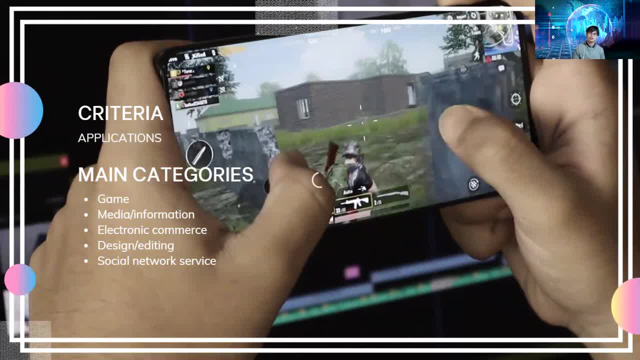 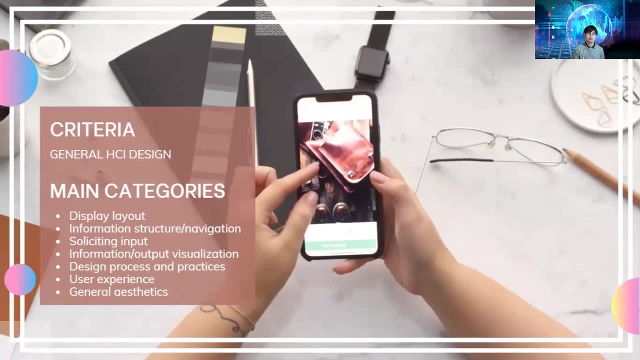 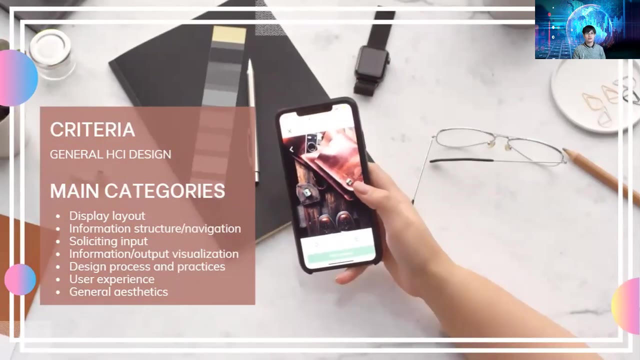 rule that will gonna form a problem, okay. so I think this is the last. okay. now this is a second to the last, okay, so after knowing the application, you must know this next criteria: the general HCI design. so in general HCI design, it just involved the display layout, the information structure and navigation, the 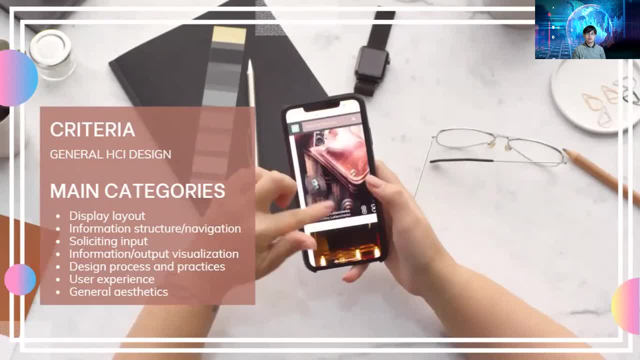 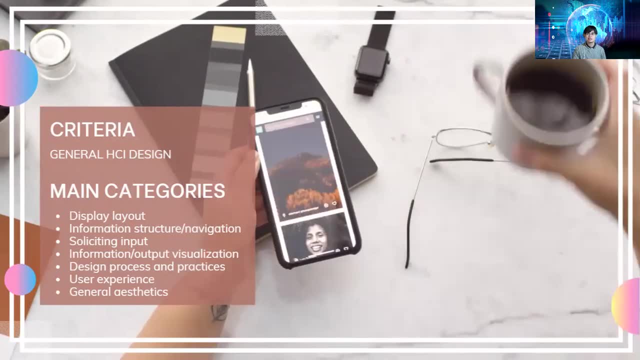 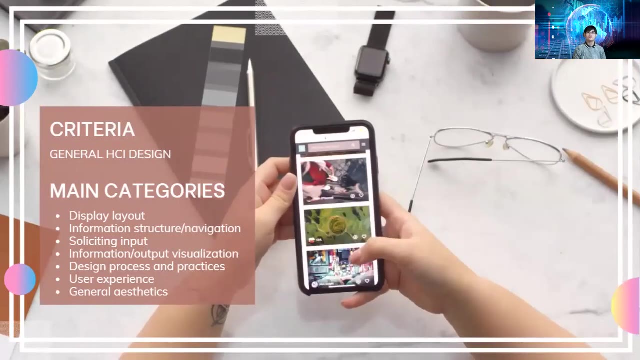 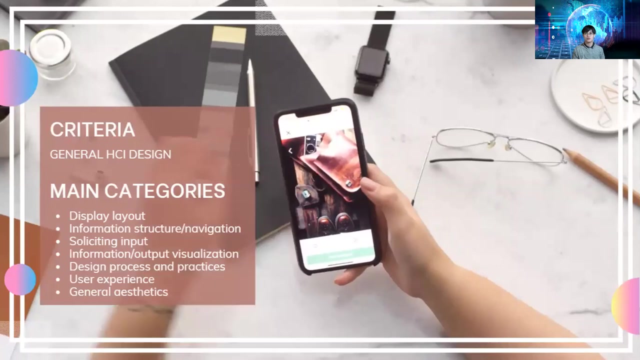 soliciting input. and as for the soliciting input, it is just the. the application is forms where it gets the data of the user. so, as you can have observed, all application have forms for you to fill out and, yeah, for you to send your data, and the information are out of. 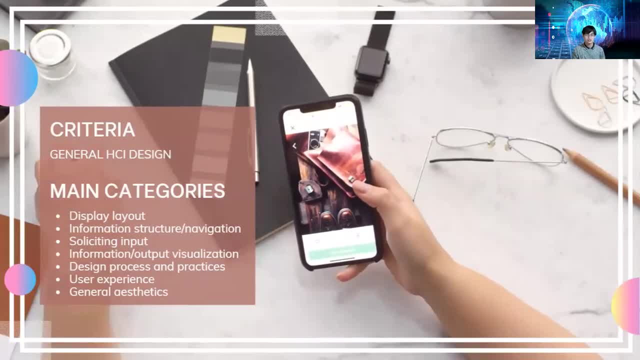 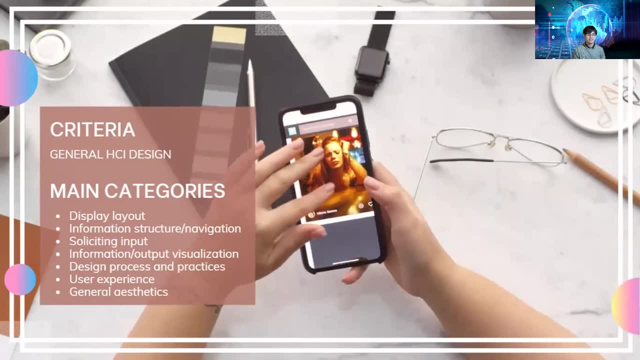 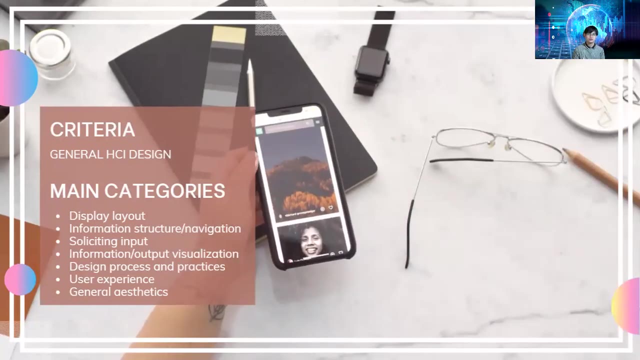 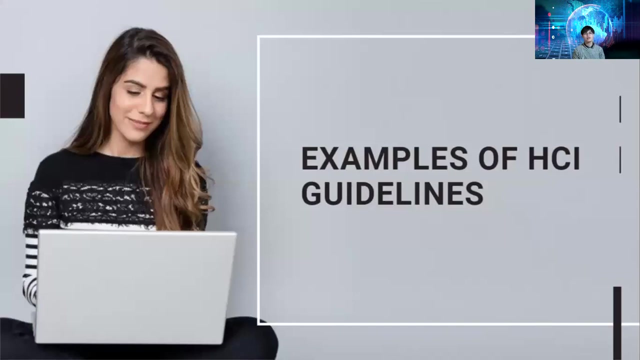 visualization very important, that is in process and practices. the user experience: okay, was it good, was it nice? and then the general aesthetics: okay, so that is the main categories of applications, the general HSA design. so those were the different criteria and the different categories when creating a really good interface. so if there are things that is. 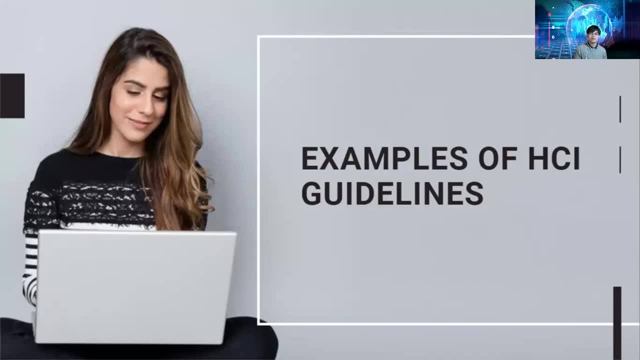 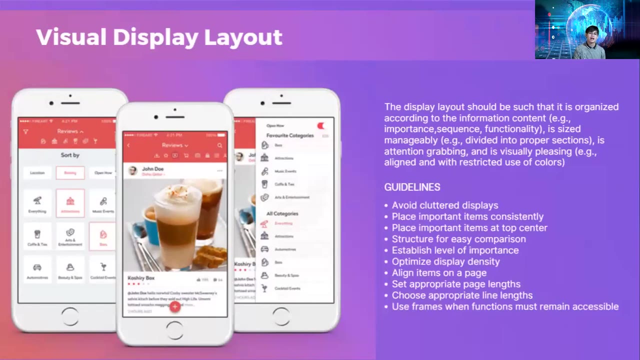 not really clear to you, you may go back, you may replay the video, then just watch it again. okay, the next topic is the examples of HSA guidelines. so what are the different examples? okay, as for the visual display layout, the display layout should be such that it is organized according to the information. 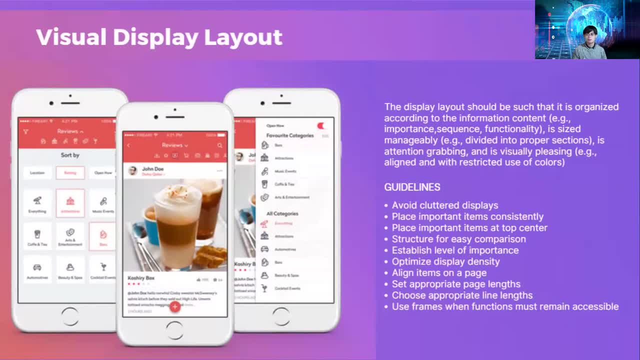 content. okay. an example: important sequence: functionality is sized manageably. okay. it is divided into proper sections. okay, and is attention grabbing and is visually pleasing. is it nice with it for the eye? is it so? does it have a really good interface? does it? are everything is aligned and with 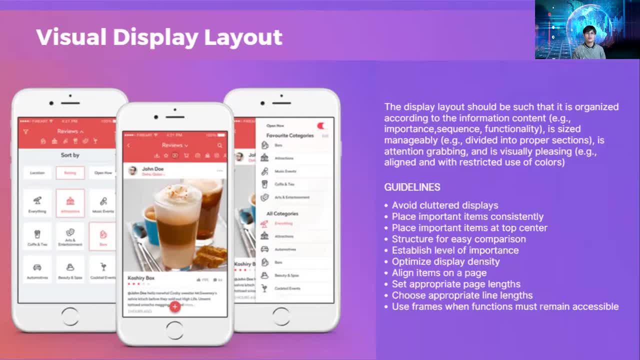 restricted use of colors, because you might use too many colors. okay, so in a visual display layout, the guidance for that would be: avoid fluttered displays. okay, imagine yourself as a user browsing this system, and then there are color displays. what? how would you feel? okay, so you might end up closing the. 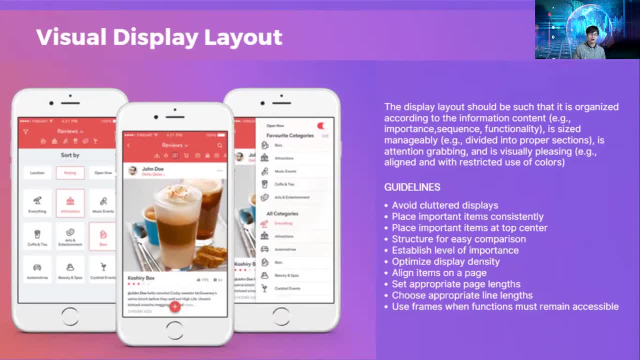 application. if there are some color displays or there are displays that you don't really like, okay, and place important items consistently, okay, and then place important items at the top center. okay. for example, what is the most important item? let's say the navigation? okay, where are you going to? 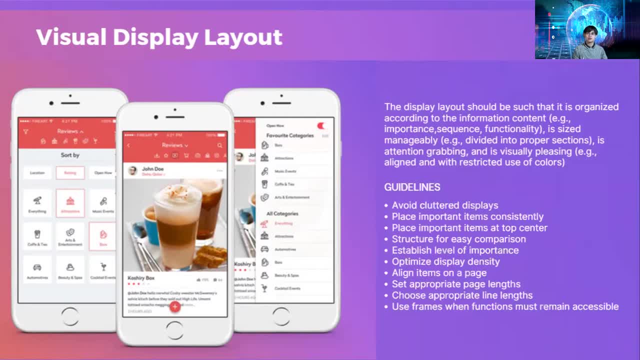 put the navigation. it should be at the top center, where in the user can easily click, it can easily navigate to it. okay, structure for easy comparison. established level of importance. so what are? this section? it is planning a section, next section of it, in the next section, next section. so you must have 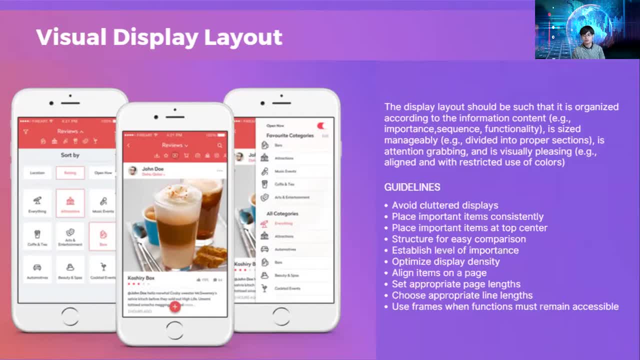 established the level of importance and then optimize display density. align items on the page you set appropriate page length. so your your page one page. should that be appropriate page length? so your your page one page, should that be appropriate page length? so your your page one page, should that be. 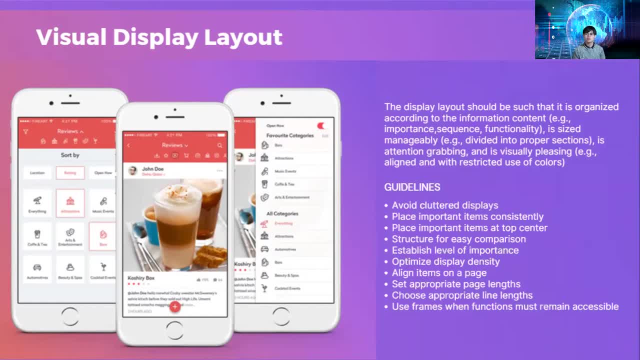 the user gonna work, you know, if there are too much information he's seen in your home page, okay, and then use frames when functions must remain accessible. so, as you can see, we have this example here. the navigation is at the right corner, okay, the items are, you know, are displayed appropriately. so the 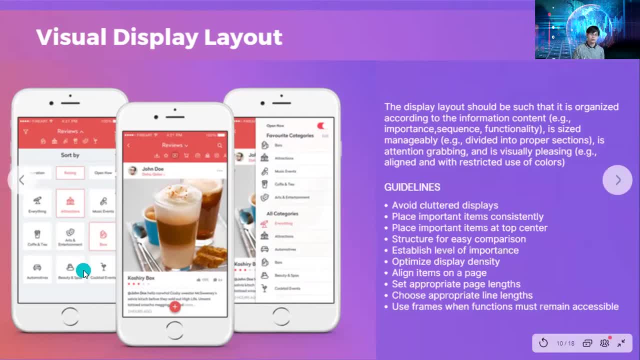 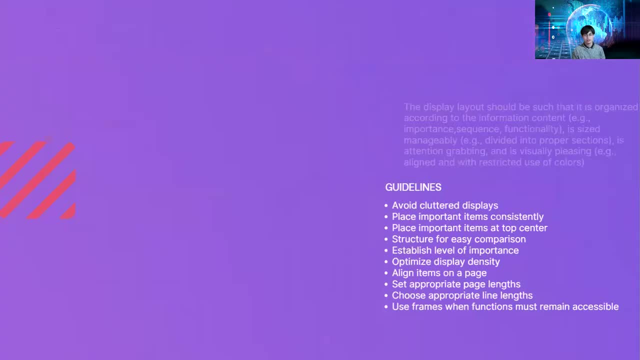 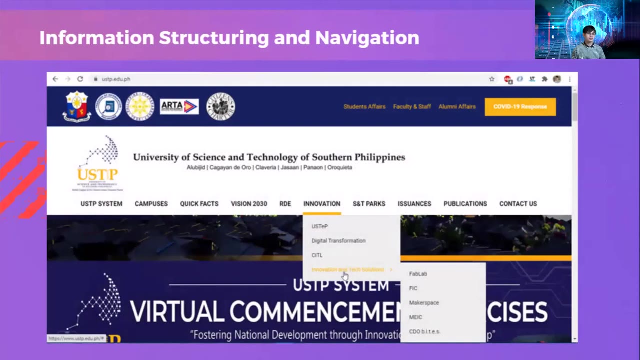 alignment is good, the colors used is good, so it should be pleasing. it should be visually pleasing information structure in navigation. this is very important whole system. we have navigation. this is very important whole system. we have noticed there are navigation, so it would be very hard for the users to you know. 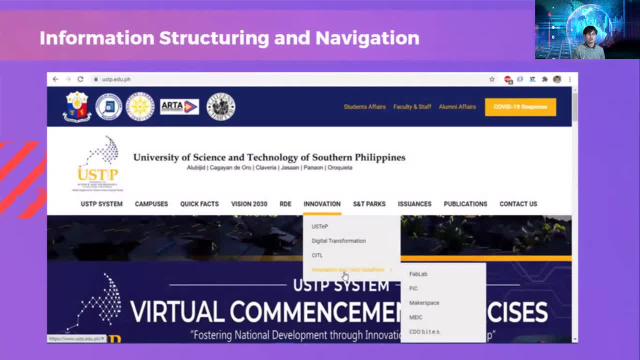 access the pages if there is no navigation being used in your system. so, as you can see, see, we have this example. okay, if the user wants to check the different campuses, you're just going to click here and then, if the user wants to contact or contact the administrators, you can actually. 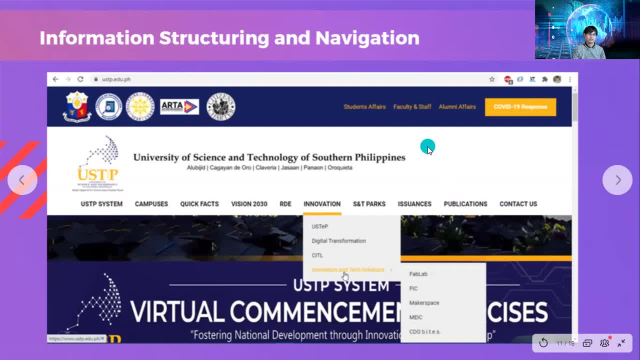 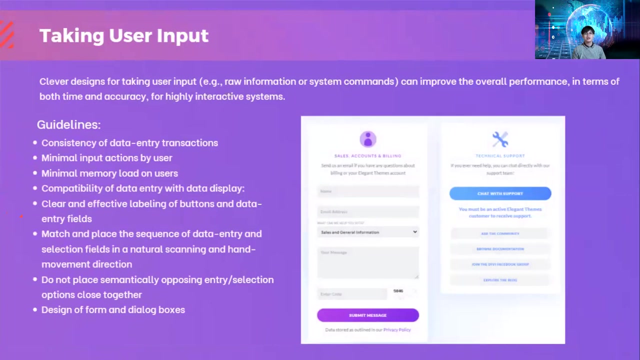 go to the contact us or check the different faculty and staff and etc. so, as this example it has, your system must be properly structured and the user must easily was able to navigate your system. okay, this is very important. there should be structuring and navigation. next, taking user input. okay, this is one of the most important thing because it would be um. 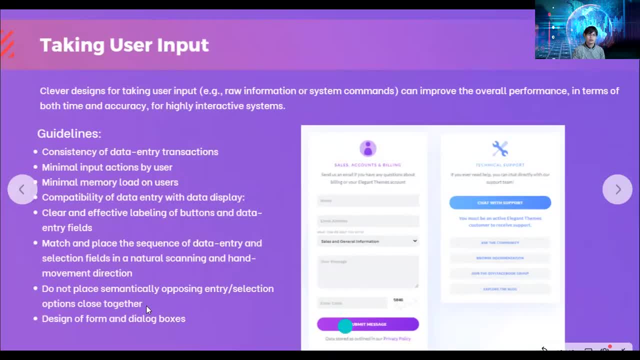 wait. okay, it would be. you know well, let's say if, if the system now details, you can see user. so, as you may have seen that the clever designs for taking user input, a row information resistance commands, can improve the overall performance in terms of both time and accuracy for highly. 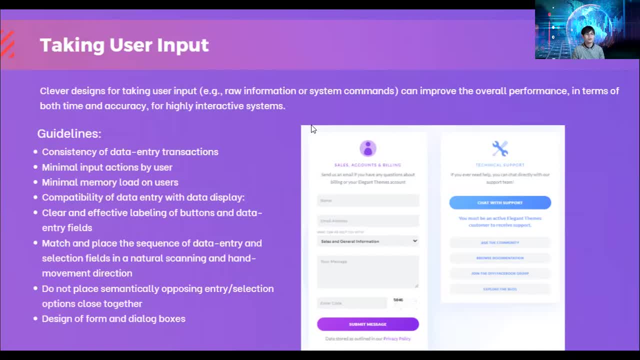 interactive systems. okay, so, of course, as you may have noticed that when you use a system, you need to create an account. so there's a form that you need to fill out and then there's a login page where you need to enter your username and password. there's a photo, and etc. okay, so what are the guidelines when? 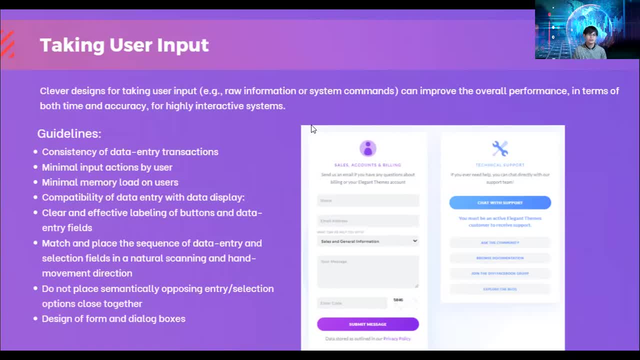 you take user input first. consistency of data entry transaction, minimal input action per user- of course we don't like, not, they can tell you like if you're out and i didn't get to happen. so minimal memory load on users. and also compatibility of data entry with data display and clear and effective labeling of. 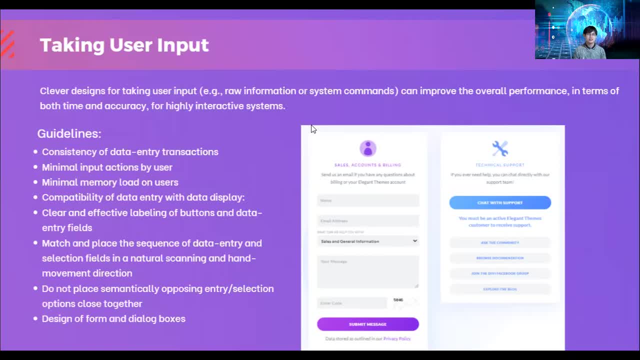 buttons and data entry fields. okay, it should be properly related. if it is for the first name, last name or email address, something like that, then match and place the segments of data entry and selection fields in natural scanning and headroom interaction and they're not placed symmetrically, opposing entry or selection. 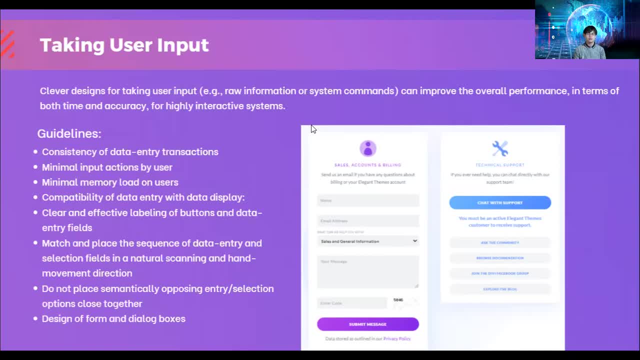 options close together, as, for example, um you, you put the um the same button, then the undo button. you must think about how by so the user in your stream number saved is undue, so na and so something like that. so it should be properly um put together. okay. 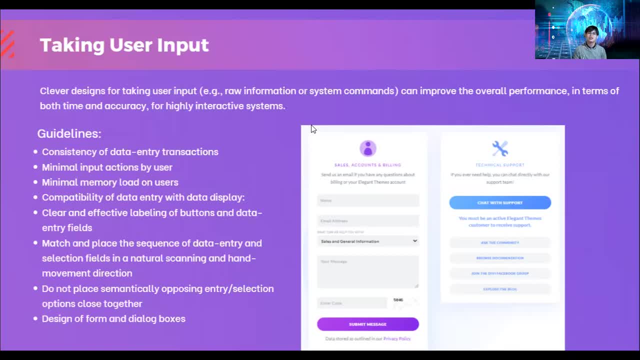 design of form and dialogue buffer. so there should be some design that is really good and pleasing for die just finding some like a design design. as you can see in here, the form has, you know, placeholder and name, email address and the shot, so the buttons are properly labeled, okay. so 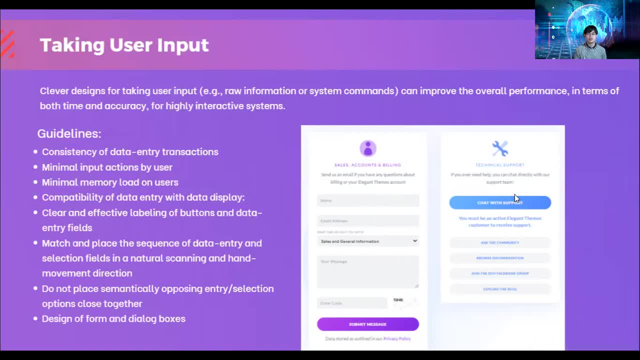 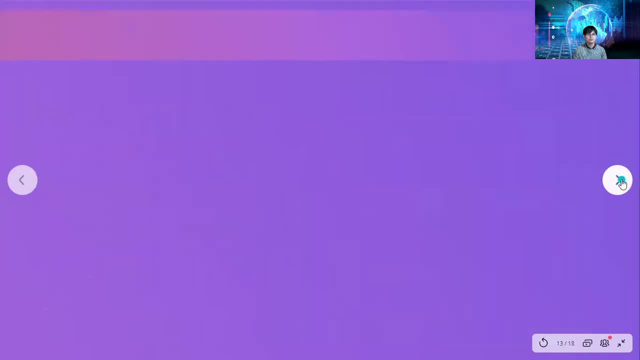 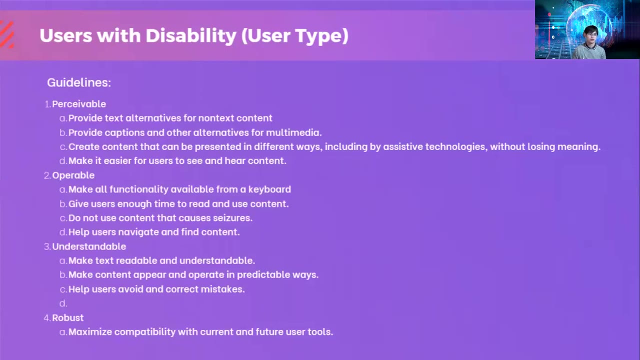 that is when you take user input. that is for the form. next, okay, users with disability. we use our text. this is a user type. okay, so when developing system and creating a system, it should be, you know, there should be options where in users with a valid disability can actually have there are. 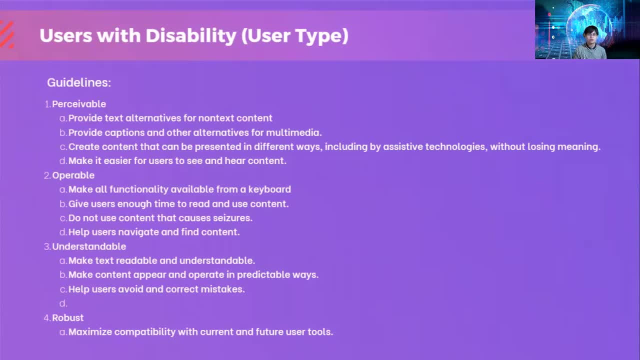 some features that they can can use. okay, so give the guidelines where that would be. it should be perceivable, meaning it. provide text alternatives for non-text content: okay, provide captions and other options, alternatives for multimedia. As you can see, YouTube now has captions, right. 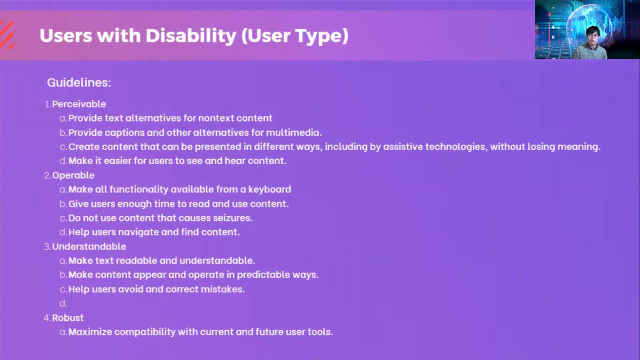 You create content that can be presented in different ways, including by assistive technologies, without losing meaning. You make it easier for users to see and hear content, so it should be perceivable And next is operable. When you say operable, 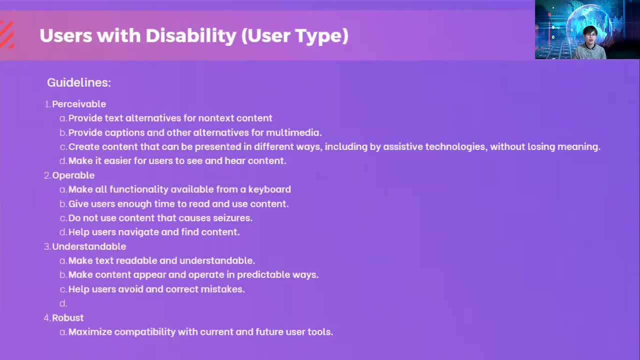 you make all functionality available from a keyboard. It's not really good that when you develop a system, there are parts that you can't make on a keyboard. Okay, So for copy and paste Ctrl-C and Ctrl-V, you have to make sure that they can do it. 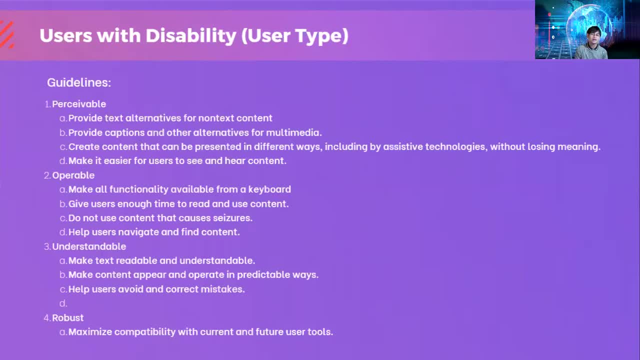 And give users enough time to read and use content. Do not use content that causes confusion, Please, or help users navigate and find content. So there should be something like something like a feature that we're gonna help the user. And next, 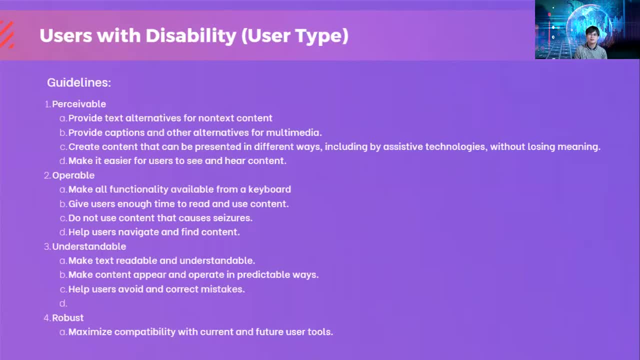 understandable- Okay. It must be user-friendly. It must be quick and easy. Make text readable and understandable- Okay. So the font sizes must not be too much small, It must not be too much large. It must be readable and understandable. Make content appear and operate in predictable ways. Help users. 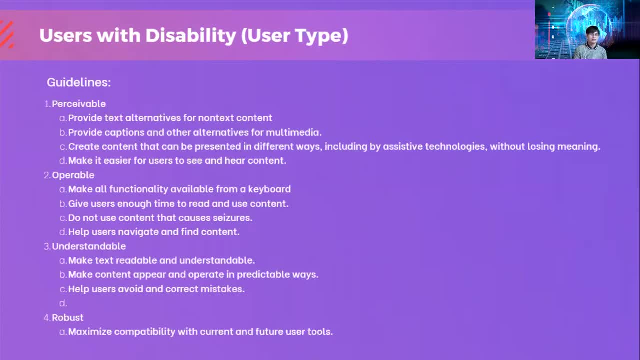 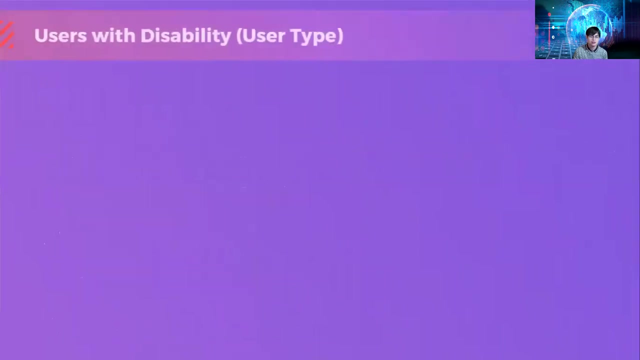 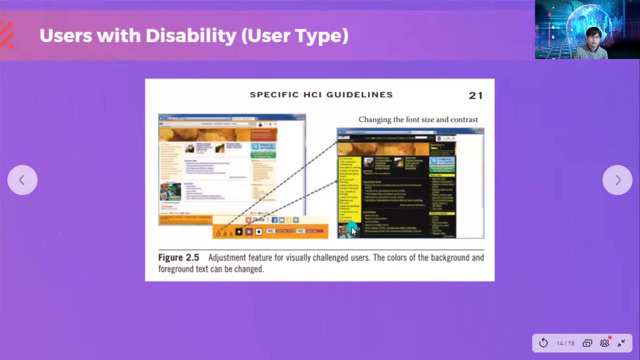 avoid incorrect mistakes, Okay. And lastly, for the users with a disability, it must be robust. You maximize capability with current and future users, too, Okay. So there are a lot of tools that you can actually use. We have this example. We have this example in here. As you can see this. 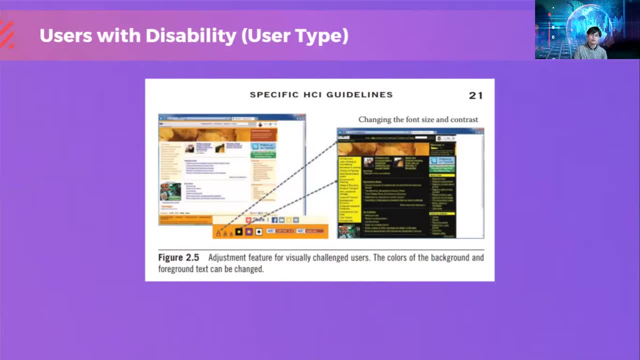 website has this option, This option for the visually challenged users, where in the user can actually change the colors of the background And the foreground- foreground. So there should be cities. There should be cities from all the time around And you have this chance to go to some of the places that you can find background. So definitely there should be tools that you're familiar with uploading and enabling useful text content from the teacher to a student or the user. If that has cost, We're all in. 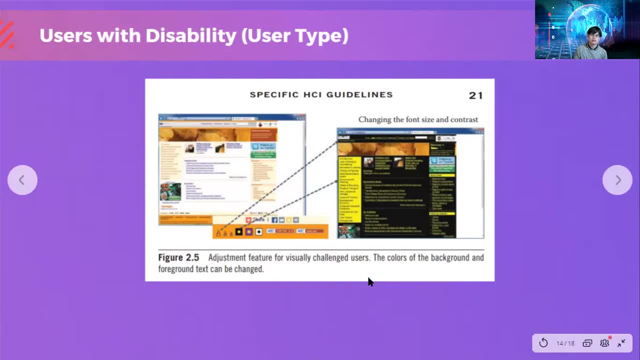 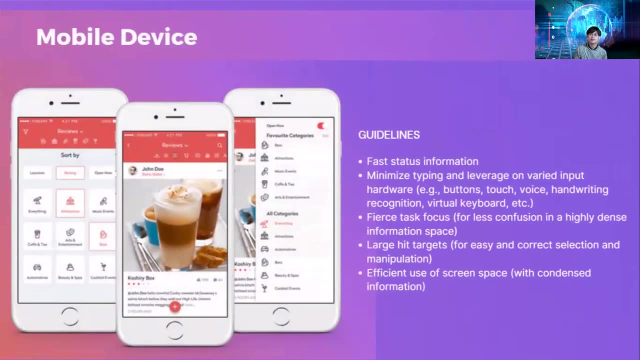 some, some features like this. okay, next is the mobile device. so, as you may have noticed, as you may have seen in all applications, that where that is a web or mobile applications, they're all mobile friendly. not everything or the system can now be used through using mobile phones. okay, as for our guidelines for 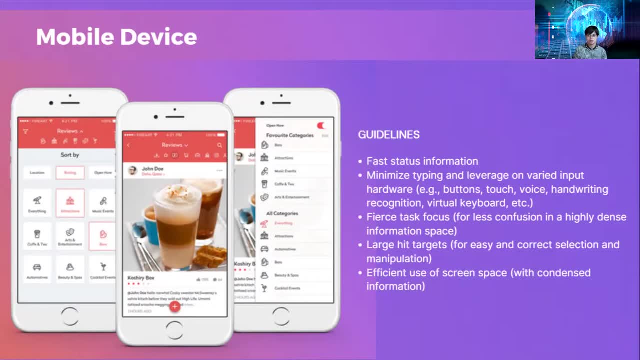 that it should be fast, status information, minimize typing and leverage on buried in bush hardware example, but on such boys handwriting recognition, vertical cable and a chest upon and then you first have to follow on. there's confusion in a highly dense information space, large hit targets for easy and correct selection and manipulation and efficient use of screen. 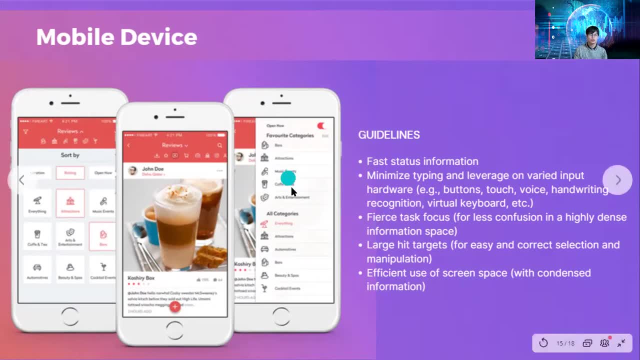 space with condensed information so you can see this example. or, as you may have noticed, on when you actually use Facebook or Messenger or Instagram, Twitter- I believe you always used that huh every day and, as you have noticed that you can actually navigate everything in real quick and easy. okay, so it should be something like that today should be. 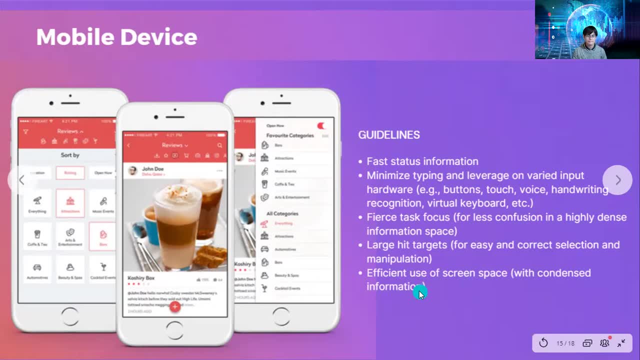 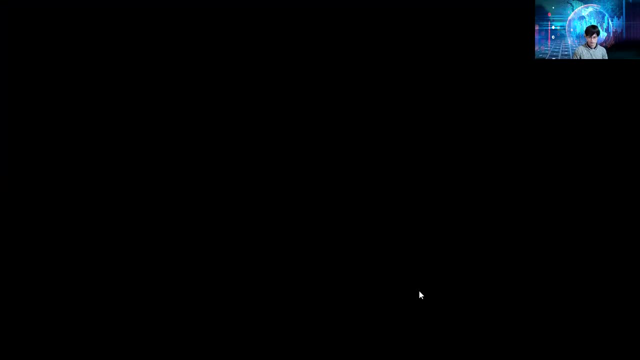 properly both on me. next big hammer. one of the most examples on best application that is everyone is using today is an economic if you have an online business. so I believe some of you have an idea what an e-commerce is, So you have been using Lazada, Shopee and a lot more. 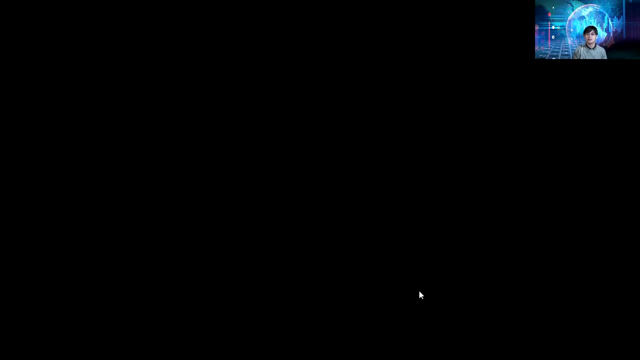 Businesses actually today are transforming into online, So that's an e-commerce, Okay. So if you want, if you have an idea and you wanted to, you know, create an e-commerce application to it, then it's your choice. Okay, so I believe you have learned something for the HSAI guidelines. 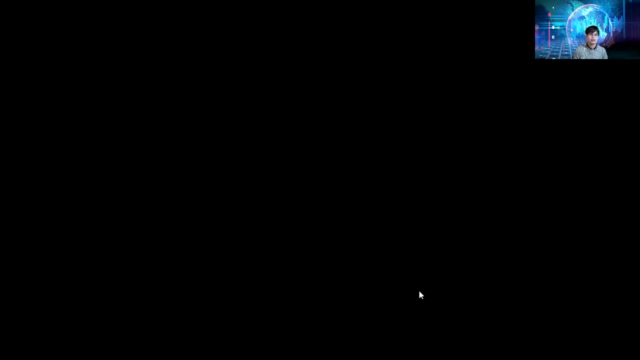 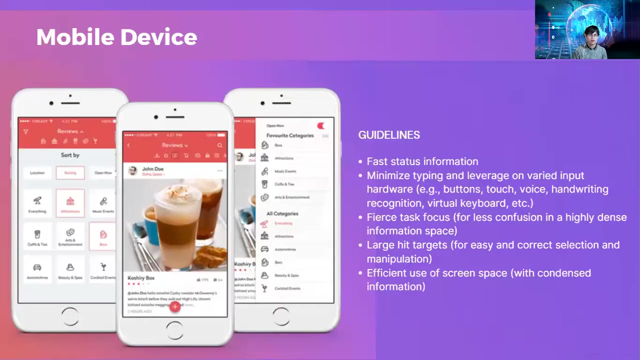 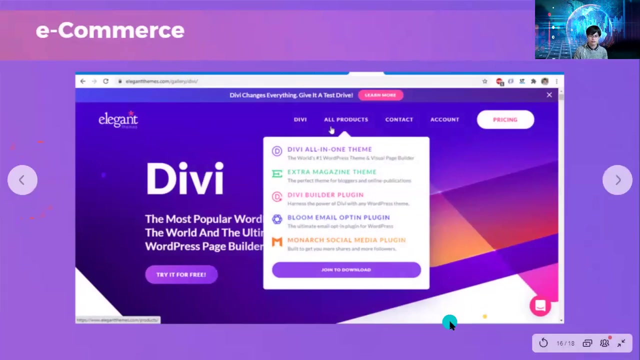 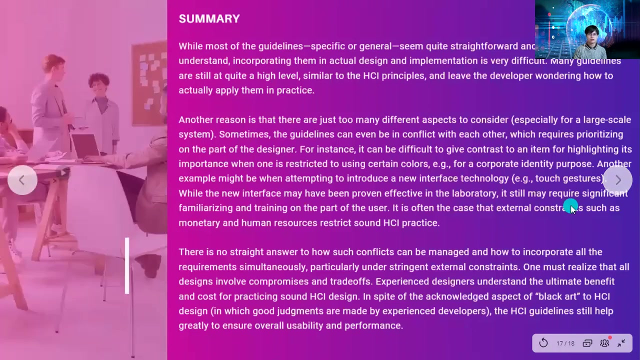 and we are now on our summary. Okay, Okay, Wait, Okay, let me go back here. Okay, this is the example of an e-commerce, because I think na-post ang screen sharing ganina. Okay, let's move on with the summary. 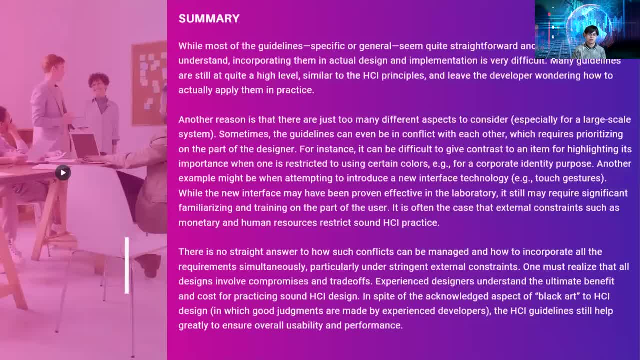 So while most of the guidelines, specific or general, seem quite straightforward and are easy to understand, incorporating them in actual design and implementation is very important. It's very difficult, It is indeed really difficult, But if you have familiar self unto it it would be more easy for you. 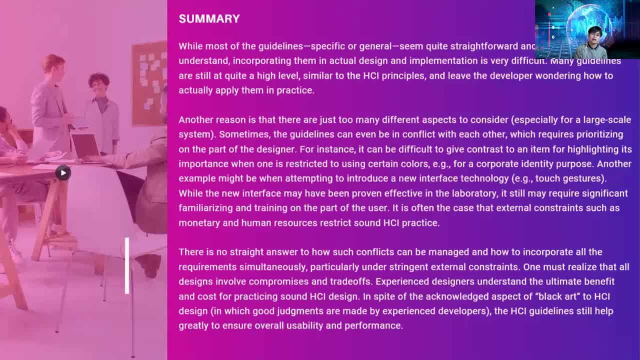 Okay, And many guidelines are still at quite a high level, similar to the HSAI principles. So if you don't know yet the different HSAI principles, then go back to our previous video in the chapter one. The HSAI principles was discussed in there. 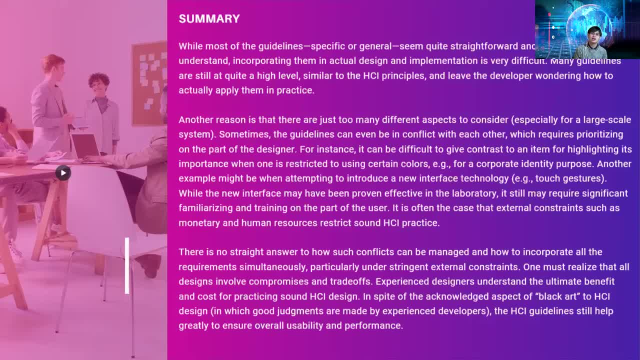 Okay, And leave the developer one comment: Okay, Okay, thank you. So now let's go to the final part, the final part of the person who is doing this And the person who are important to me. The last thing is: how is the interface on a company? 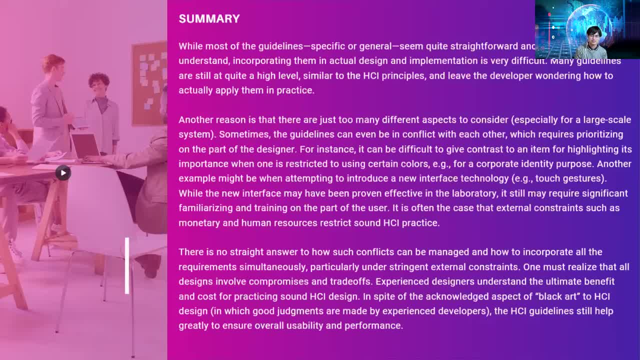 how is the interface on a company and how will the interface on a company run properly? Okay, So that's the first thing. Most of us, as designers, need to know: how to use the interface. We need to know how to use the interface properly. 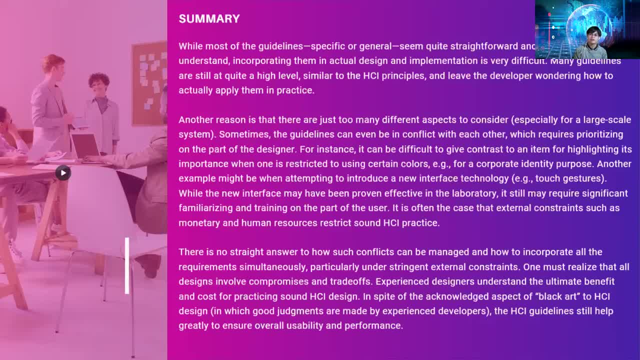 One thing that I would tell you is that most of us have a tech experience that requires to have the interface on a company. So that's a lot of time and effort to give you the guide to have the interface on a company, So you need to get that in your mind. 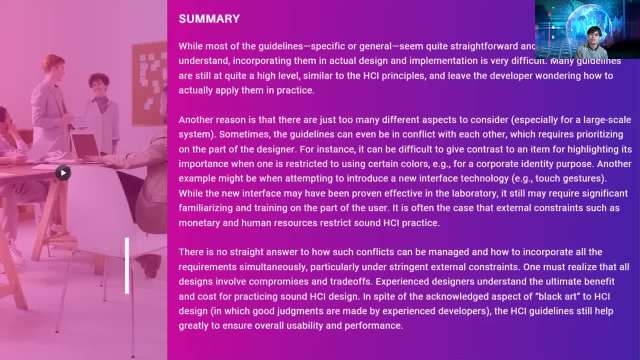 Okay. So, for example, if you have a company, because you're the one who are going to design your system, For instance, it can be difficult to give contrast to an item for highlighting its importance when one is restricted to using certain colors, For example, for a corporate identity. 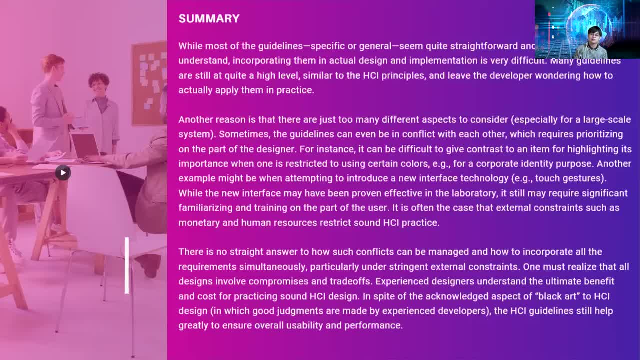 purple. Another example might be when attempting to introduce a new interface technology or touch gestures. While the new interface may have been proven effective in the laboratory, it still may require significant familiarizing and training on the part of the user. It is often the case that external